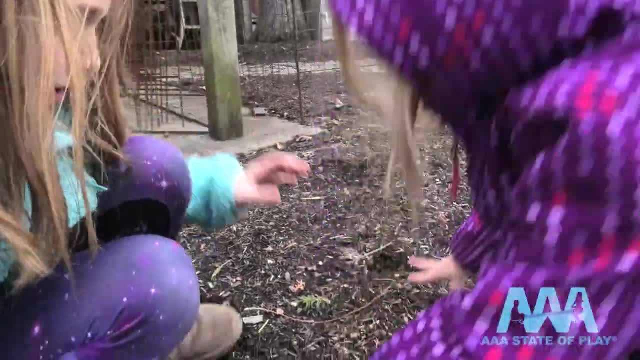 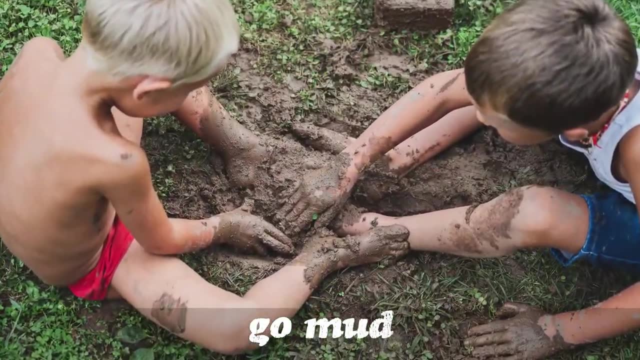 Watch the plants grow, transplant, then nurture their flowers or produce gardens all spring and summer. Perfect for learning and maybe eating. And while they have their hands in the mud, kids can play in the mud- There's usually plenty of it in the spring. 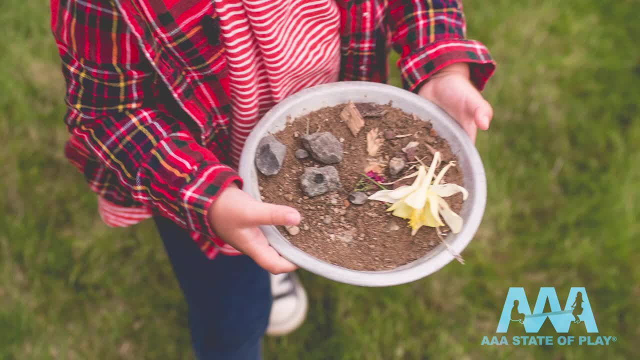 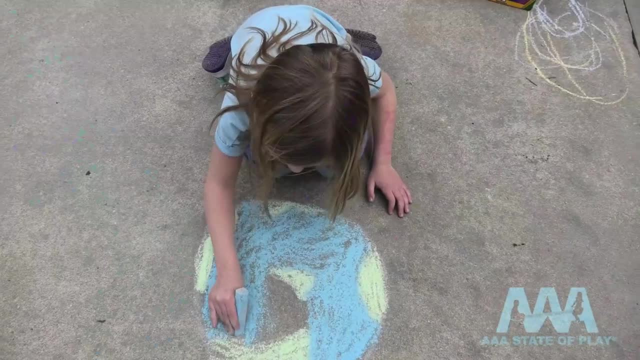 Mud, bakery, mud art, dirt can be good, clean, fun, but you may want to have a hose nearby. Children and chalk are a natural Chalk. in the classroom- boring Chalk art outside awesome. It's a simple and creative way to color their world with images. 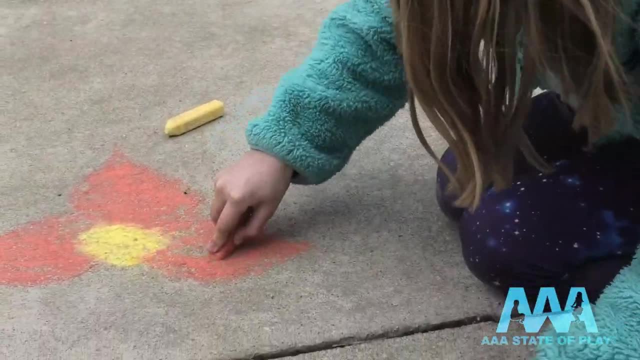 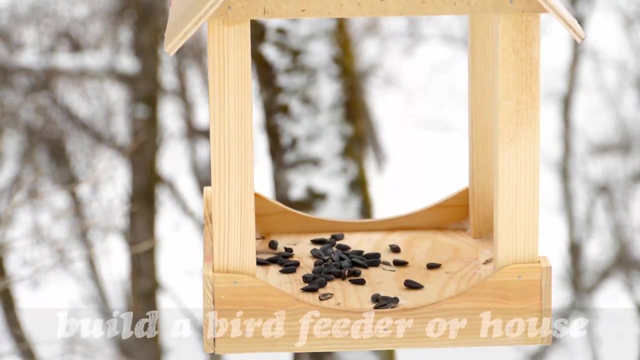 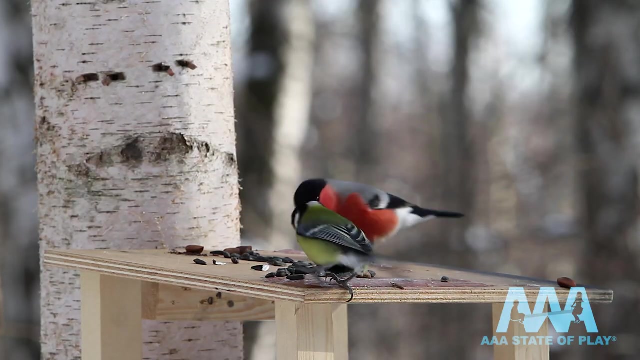 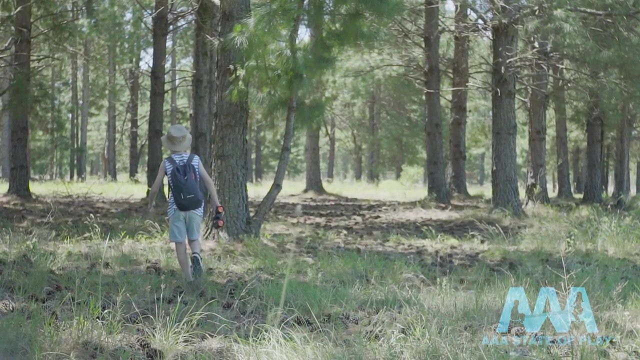 Make sure you have plenty of colors as kids channel their inner Picasso. Only this art is easy to clean and wash off. Build a bird feeder or bird house. It gives children a true hands-on experience that can nurture them and nurture nature. This springtime activity could grow an interest in further learning and exploration and greater appreciation for wildlife. 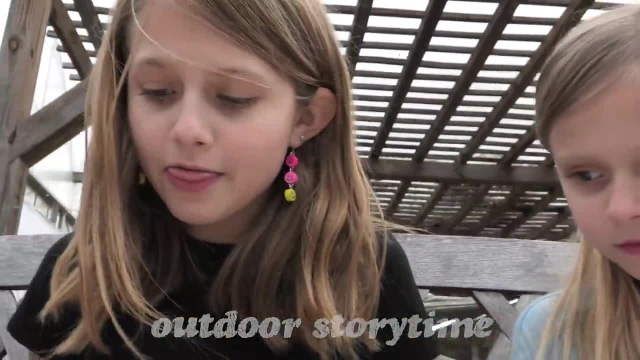 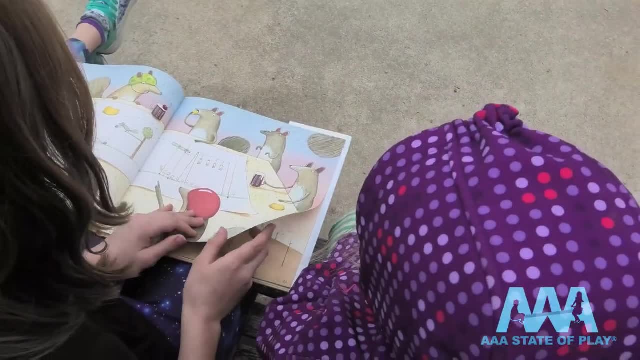 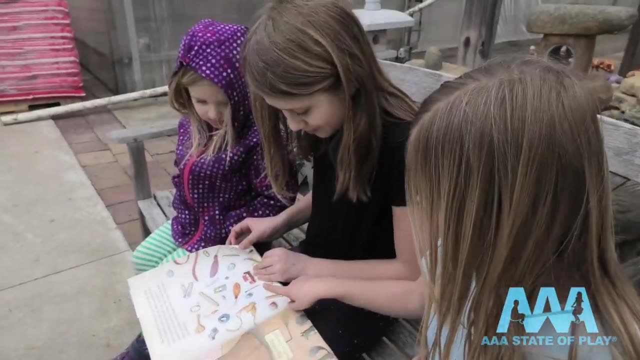 But the squirrels were determined, They devised a plan And this time they took all the food from the bird feeders. Outdoor storytime can be enriching. It's a great mix: Sunlight and stories You can read to your children. Maybe they read to you or each other. 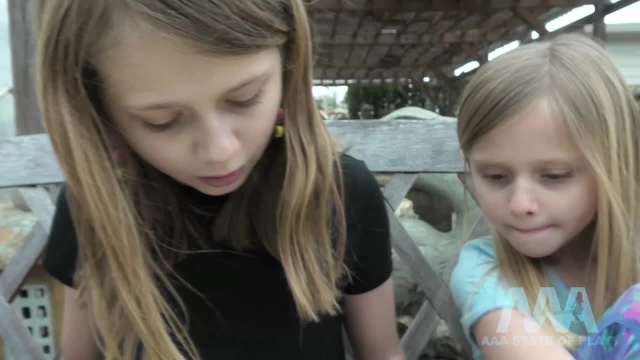 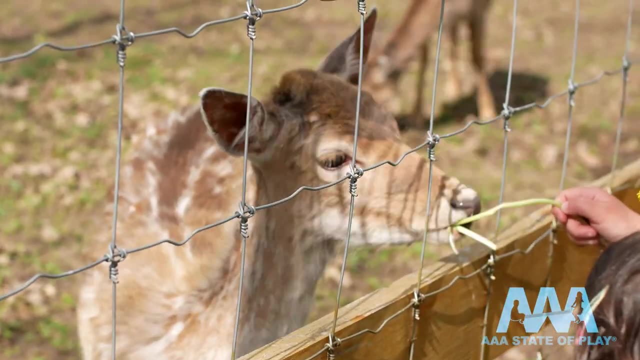 A typical indoor activity gets a real breath of fresh air. How about a trip to see something a little bigger? Springtime is a perfect time to get back to the zoo, Maybe even a local animal farm or dairy farm. Make your own bubble blowing mix. 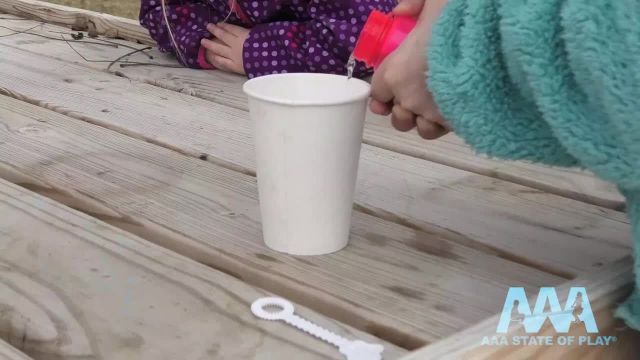 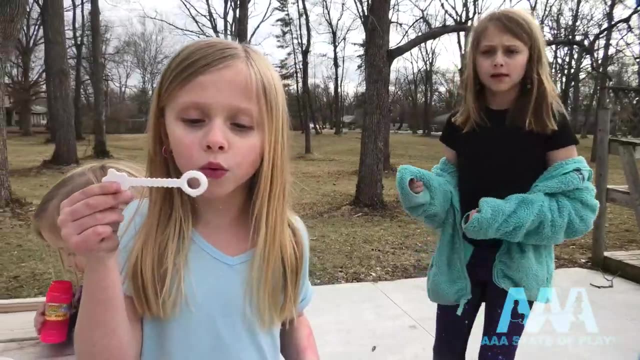 Children can build and blow a better bubble by mixing their own Bubble. recipes on the internet usually use a mix of water, dish soap and corn syrup or glycerin. Mix, blow, chase, burst and repeat. Arrange a scavenger hunt. 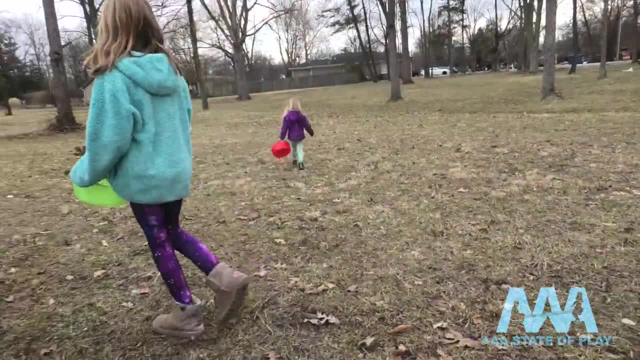 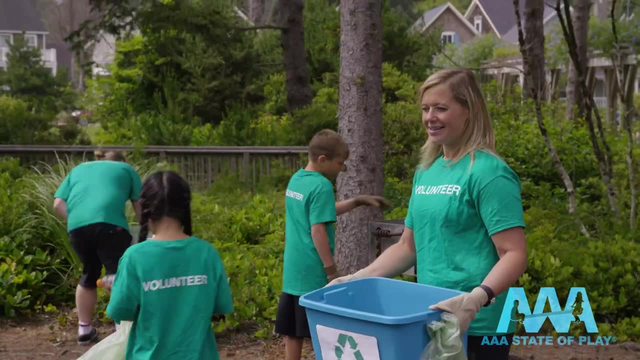 Children only need a pail or bucket and a goal of something to gather. Send kids out to hunt for specific items, bugs or pieces of nature. You can expand on that and turn the hunt into a community service. with a neighborhood cleanup And a clean earth makes for another great outdoor activity. 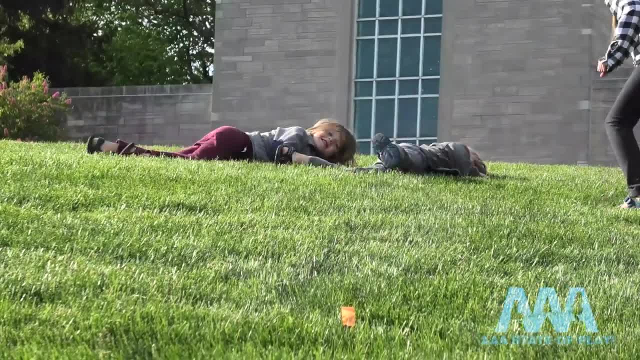 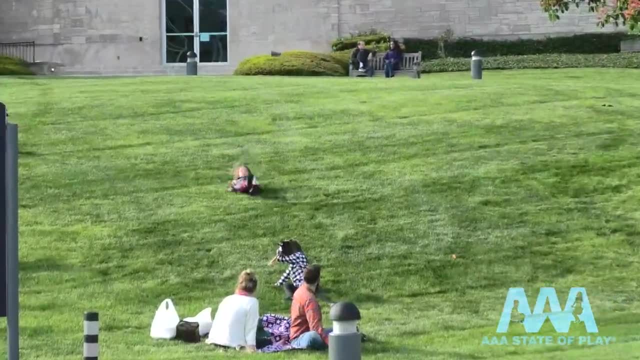 In the spring, find a hillside, even a small one, and roll rumble, tumble and stumble downhill. What better ways to spend spring days outside? Let's go.